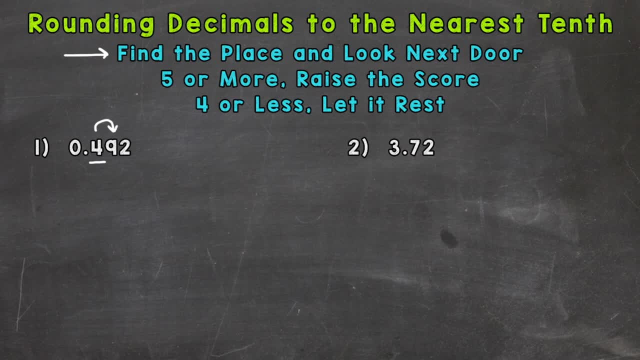 next door and it's always going to be to the right, always to the right. So we have a nine next door. so we need to determine if we round up or stay the same When we round. essentially, we're just saying: is this number closer to four tenths rounding and staying the same, or is it closer? 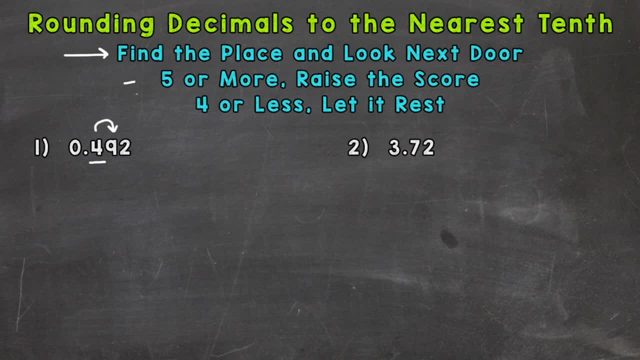 to five tenths, rounding up. So is that nine, five or more, or four or less? So a nine is obviously more than five. so five or more raise the score. so we round up to five tenths. That's our rounded answer. So that number 492 thousandths is closer to, or rounds to, five tenths. 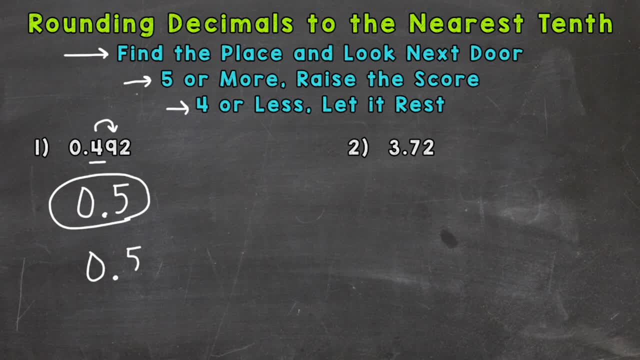 Now, when we round whole numbers, we change all the digits to the right to zeros. When it comes to decimals, you don't need these zeros here because they're just placeholder zeros. They don't hold or change any numbers value, So we can kind of cut those off and just write five. 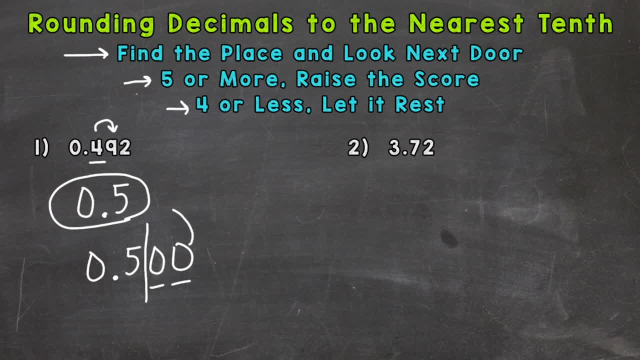 tenths, Now five hundred thousandths. that number there with the zeros is equivalent to five tenths. but again, you don't need those zeros. Let's move to number two, where we have three and seventy two hundredths. So we need to find the place that we're rounding to the tenths and we have a seven. 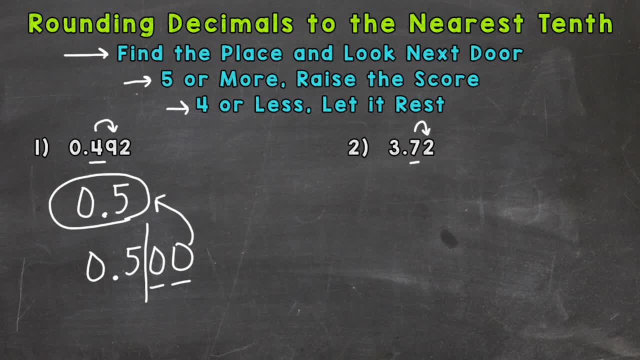 Let's look next door. We have a two, so is that five or more? And we round up, or is it four or less? And that seven stays the same. Well, two is four or less, So we let that seven rest. so we stay the same here. 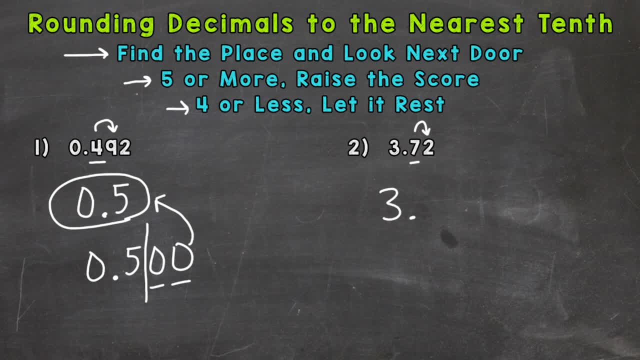 So three and seventy two hundredths rounds to three and seven tenths. It's closer to three and seven tenths than it is to rounding up to three and eight tenths. So this is our answer here, And remember we can cut that decimal off after the rounded place. 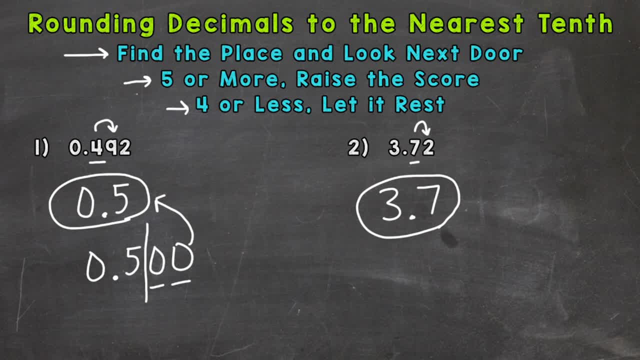 We don't need any zeros To the right. So there you have it. There's how you round decimals to the nearest tenth. Now I have other videos as far as rounding goes. I dropped all of those links down in the description. I hope this helped. Thanks so much for watching. Until next time, Peace.